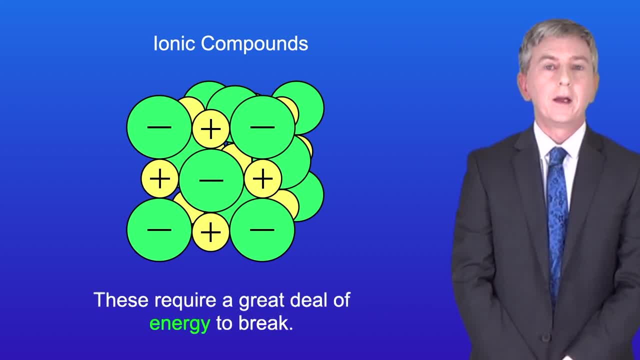 of attraction. These require a great deal of energy to break and this means that ionic substances have got very high melting and boiling points. For example, the boiling point of sodium chloride is over 1400 degrees Celsius. I'm showing you here the boiling points of some covalent 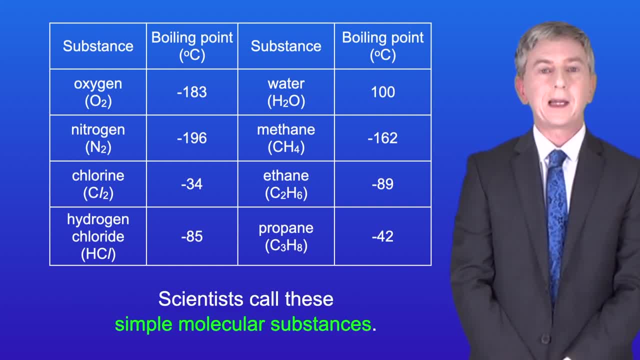 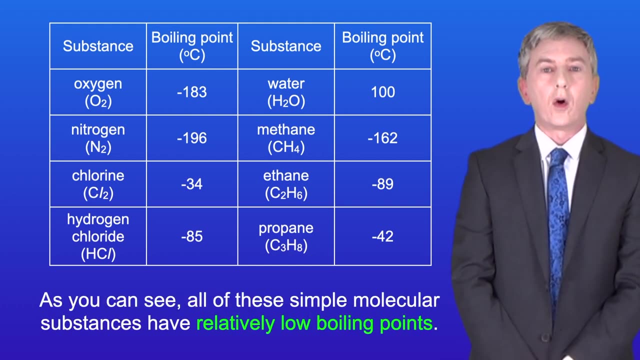 substances. Now scientists call these simple molecular substances. What that means is that they consist of relatively small molecules, and each molecule has a fixed number of atoms. Giant covalent substances such as graphite would not fall into this category. As you can see, all of 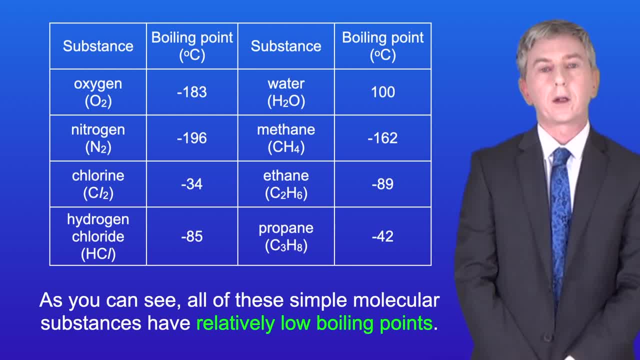 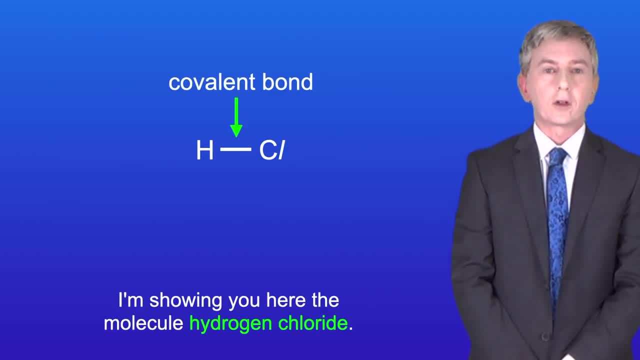 these simple molecular substances are made up of a very high melting point of sodium chloride. The molecular substances have got relatively low boiling points. To explain this, we need to look at the bonding in these substances. I'm showing you here the molecule hydrogen chloride In hydrogen. 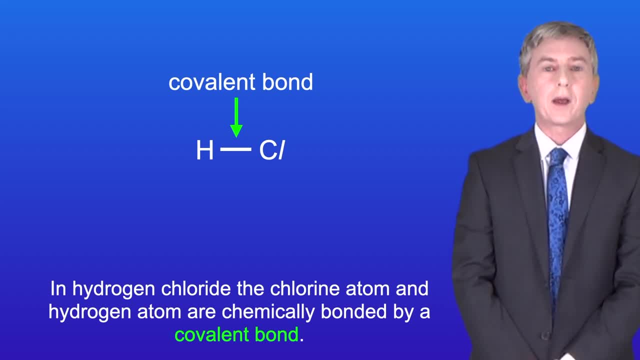 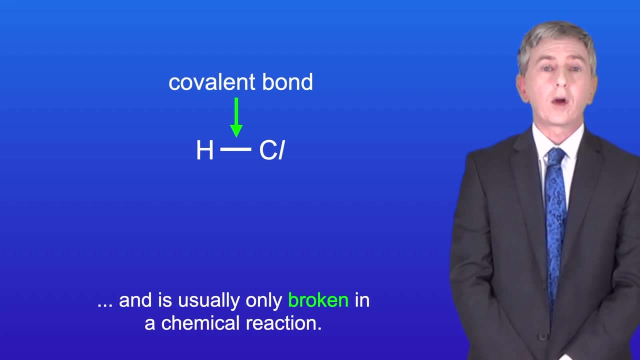 chloride, the chlorine atom and hydrogen atom are chemically bonded by a covalent bond. You need to remember that a covalent bond is extremely strong and is usually only broken in a chemical reaction. Covalent bonds are not affected at all when a substance boils. Now as well as covalent. 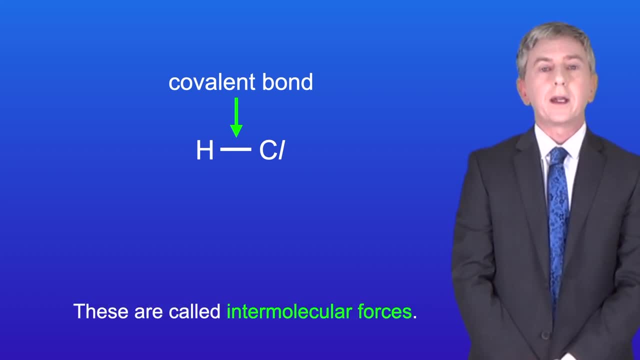 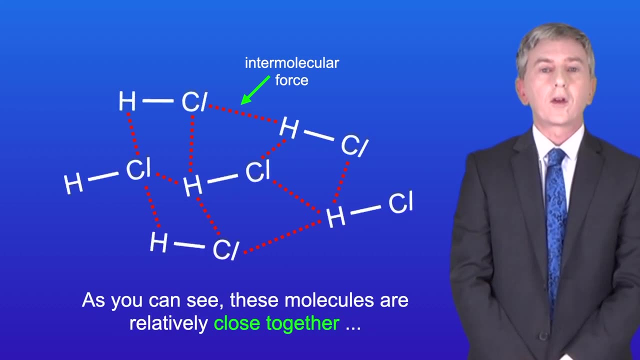 bonds. we also need to consider another type of bonding. These are called intermolecular forces. I'm showing you here a number of hydrogen chloride molecules. As you can see, these molecules are relatively close together, so this could be, in the liquid form, Intermolecular forces. 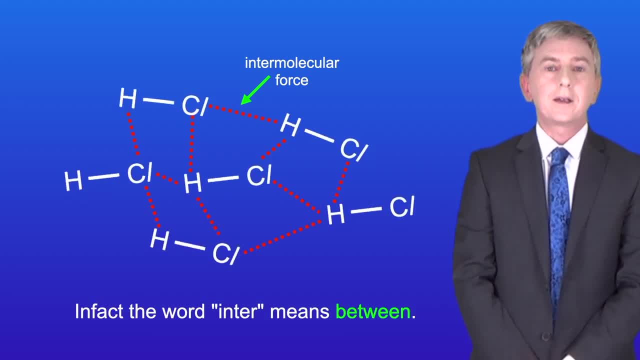 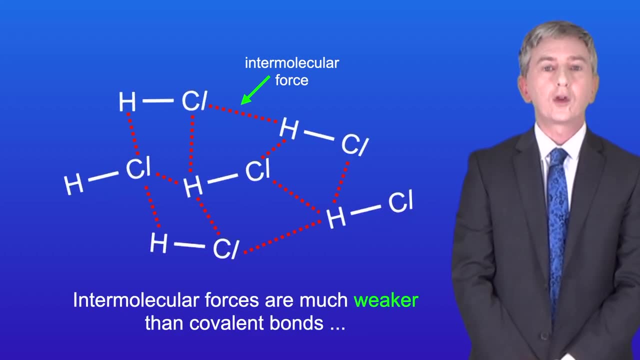 of attraction act between molecules and in fact the word inter means between. I'm showing the intermolecular forces as dotted lines. Intermolecular forces are much weaker than covalent bonds and are easily broken, for example by high temperature. When we heat a simple molecular substance, this causes the molecules to move. 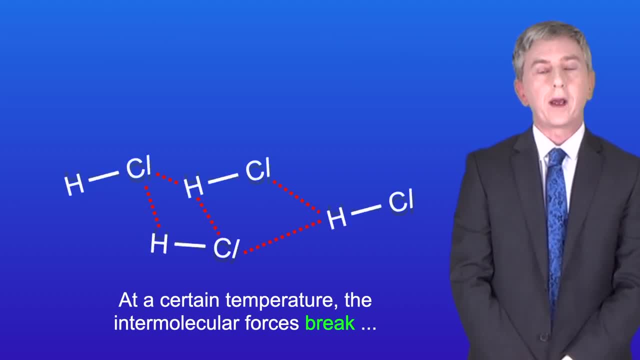 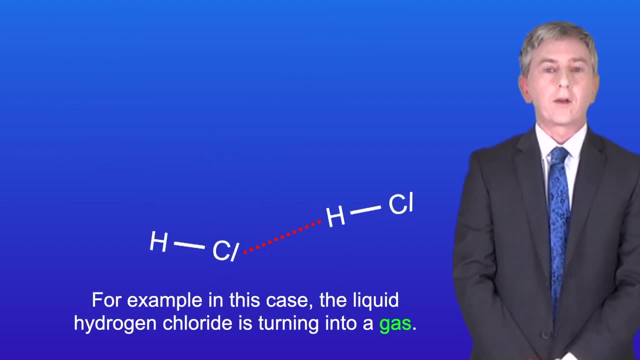 faster. At a certain temperature, the intermolecular forces break and this allows the molecules to move away from each other. So, for example, in this case, the liquid hydrogen chloride is turning into a gas Now, as we saw before, simple molecular substances such as hydrogen 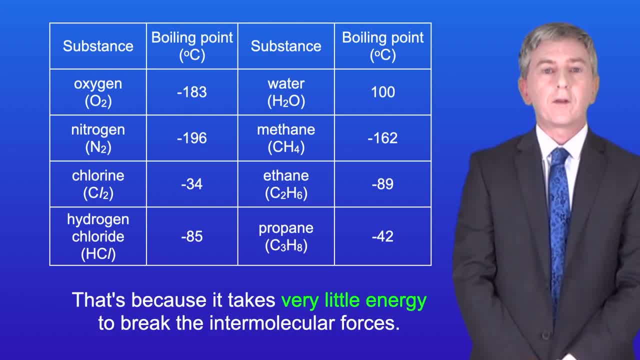 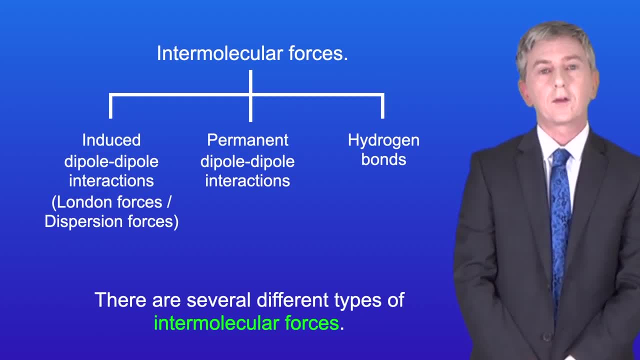 chloride have got low boiling points, And that's because it takes very little energy to break the intermolecular forces. OK, now there are several different types of intermolecular forces. We've got induced dipole-dipole interactions, which are also